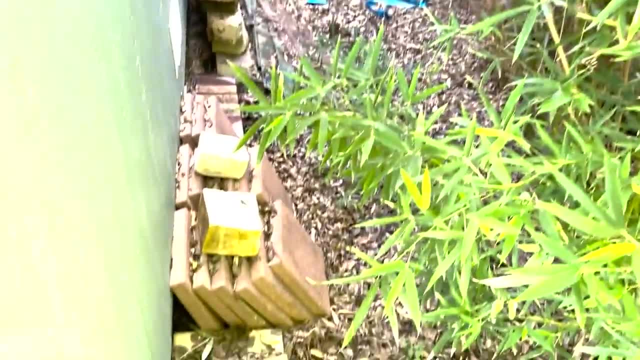 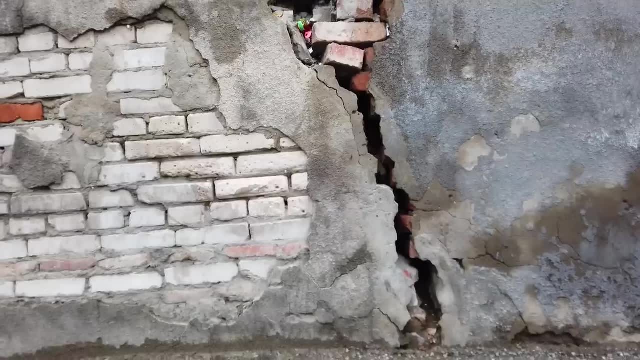 in a landscaping project someday, but their most likely future is to sit here in the shady purgatory for all of eternity. Unfortunately, buildings and other structures are a little different. Mainly, they're large enough that one part could move relative to the other parts. 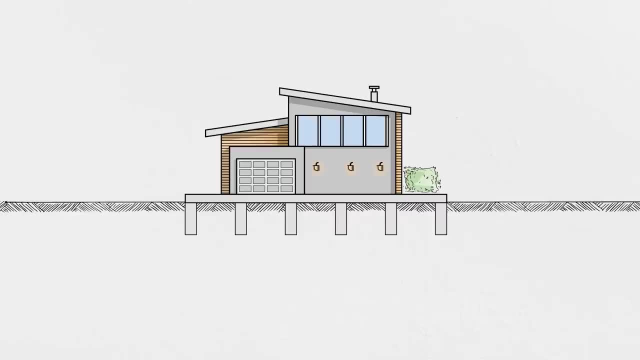 a phenomenon we call differential movement. When you move one piece of any thing relative to the rest of it, you introduce stress, And if the stress is greater than the inherent strength of the thing, that thing will pull itself apart. It happens all the time. 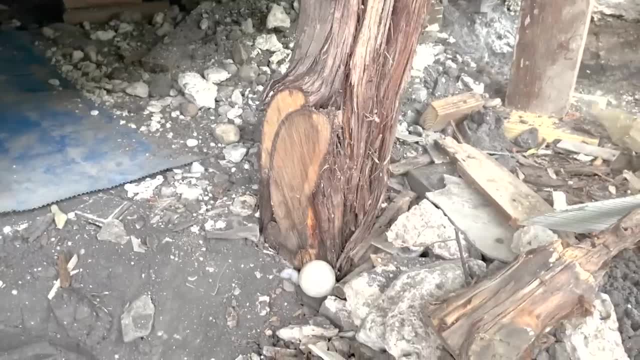 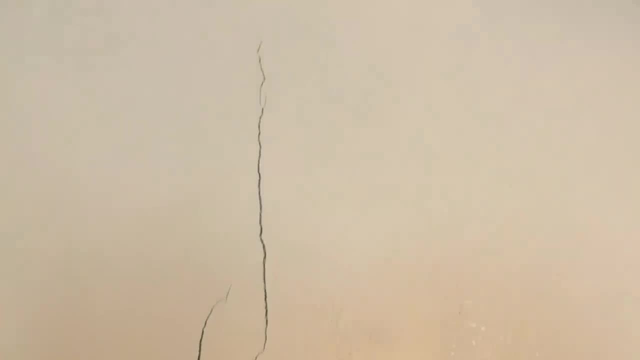 all around the world, including right here in my own house. When one of these piers settles or heaves more than the others, all the stuff it supports tries to move too. But door frames, drywall and ceramic tile work much better and last much longer when the surrounding structure. 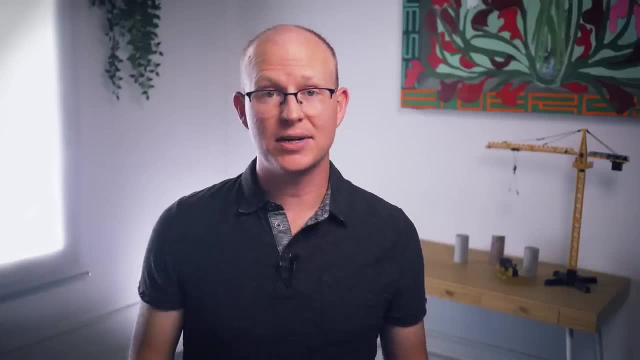 stays put. There are many kinds of foundations used for the various structures in our built environment, But before we dive into how they work, I think it will be helpful to first talk about what they're up against, or actually down against, Of course, buildings are. heavy, and one of the most important jobs of a foundation is to evenly distribute that weight into the subsurface as downward pressure. Soil isn't infinitely strong against vertical loads. It can fail, just like any other component of a structural system, When the forces are high. 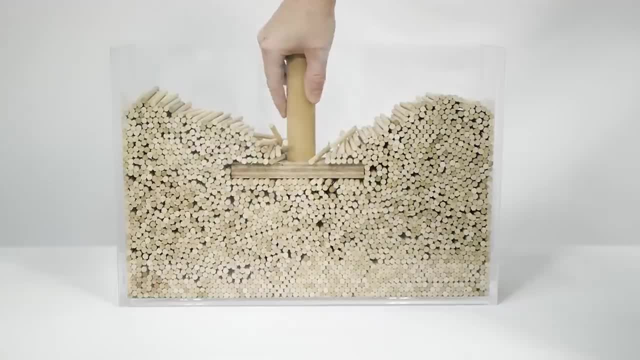 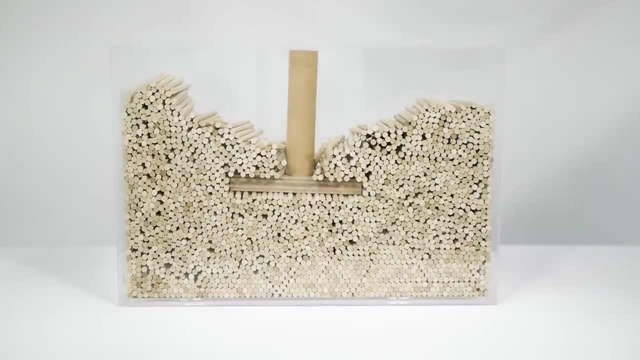 enough to shear through soil particles. we call it a bearing failure. The soil directly below the load is forced downward, pushing the rest of the soil to either side, eventually bulging up around the edges. Even if the subsurface doesn't fall on top of the other side, it's still going to fall. 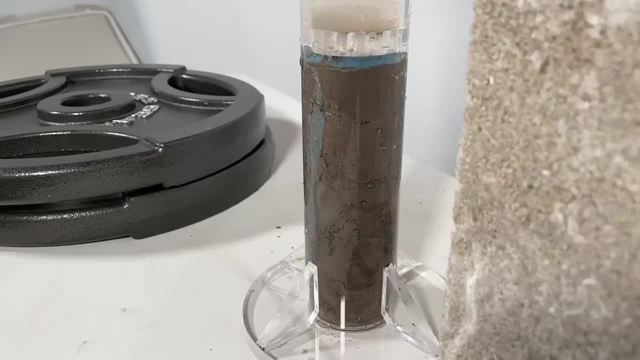 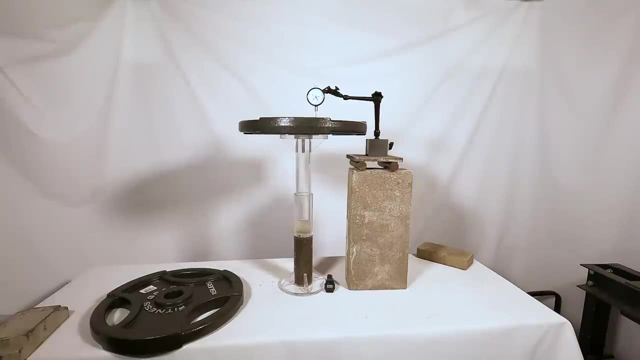 on top of the other side. This happens when the particles are compressed more closely together, and it usually takes place over a longer period of time. I have a video all about settlement that you can check out after this. So job number one of a foundation is to distribute the downward 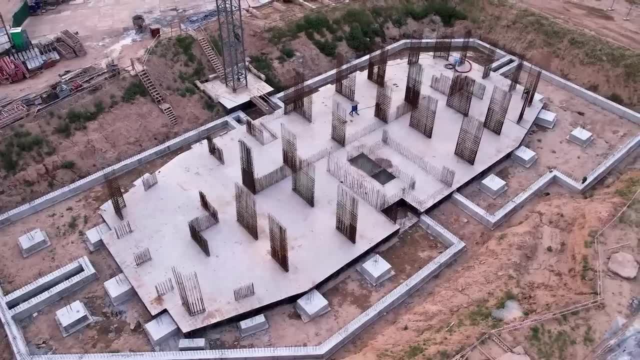 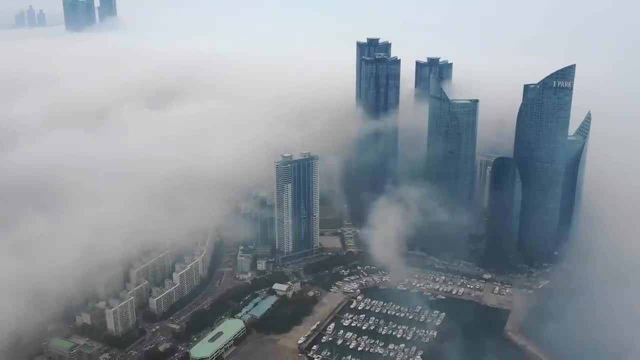 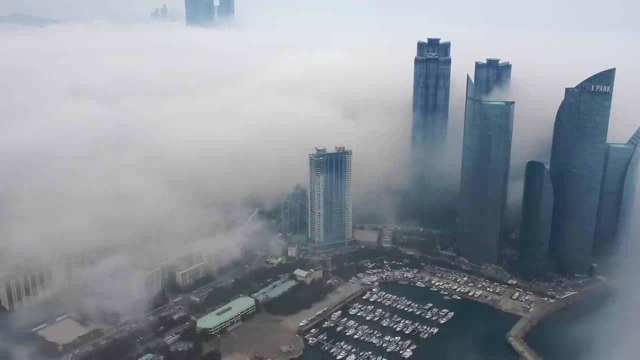 force of a structure over a large enough area to reduce the bearing pressure and avoid shear failures or excessive settlement. Structural loads don't just come from gravity. Wind can exert tremendous and rapidly fluctuating pressure on a large structure, but it can also cause damage to the structure, pushing it horizontally and even creating uplift like the wing of an. 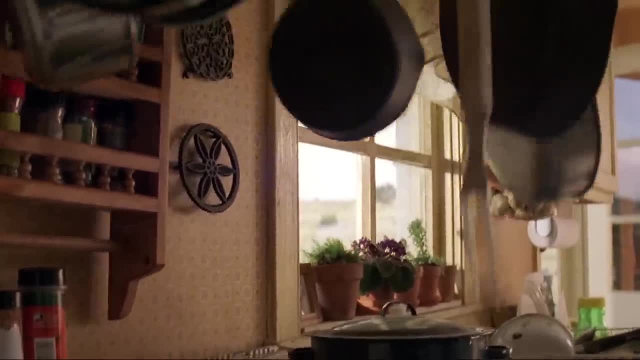 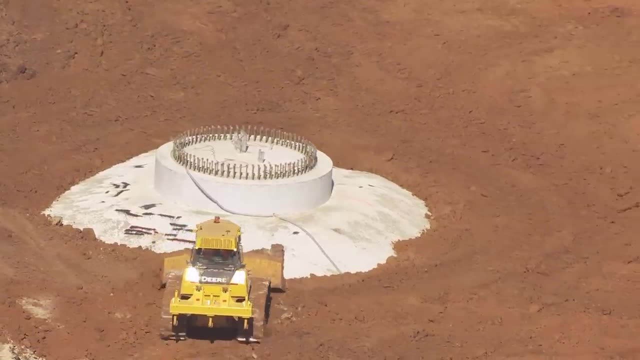 airplane. Earthquakes also create loads on structures, shifting and shaking them with very little warning. Just like the normal weight of a structure, these loads must also be resisted by a foundation to prevent it from lifting or sliding along the ground. That's job number two. 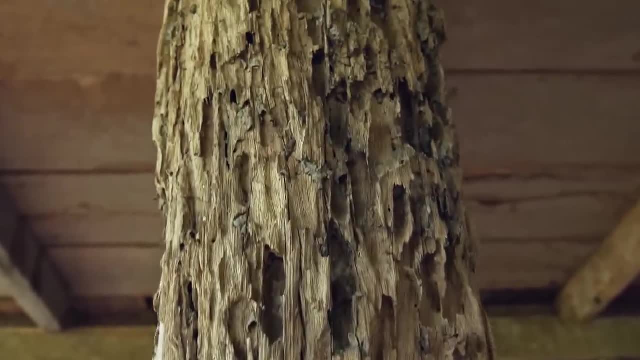 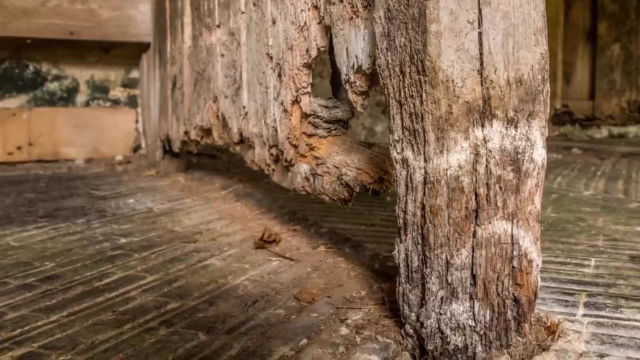 Speaking of the ground, it's not the most hospitable place for many building materials. It has bugs like termites that can eat away at wooden members over time, reducing their strength. It also has moisture that can lead to mold and rot. My house was built in the 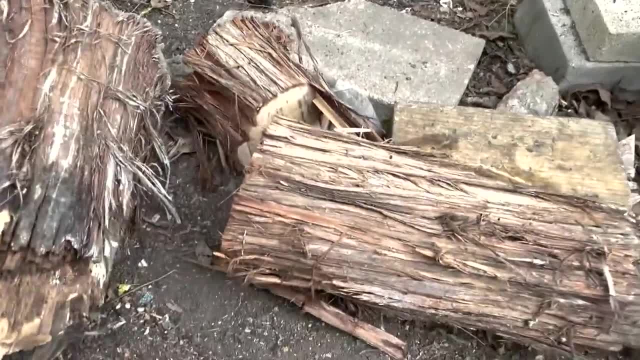 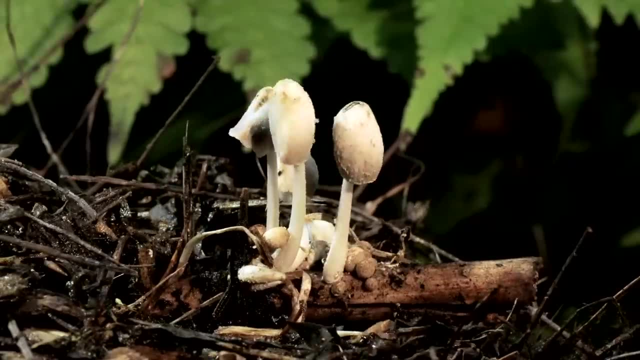 1940s on top of cedar piers. This is a wood species that is naturally resistant to bugs and fungi, but not completely immune to them, as you can see. So job number three of a foundation is to resist the effects of long-term degradation and decay that come from our tiny. biological neighbors. Another problem with the ground is that soil isn't really as static as we think. Freezing isn't usually a problem for me in central Texas, but many places in the world see temperatures that rise and fall below the freezing point of water tens or 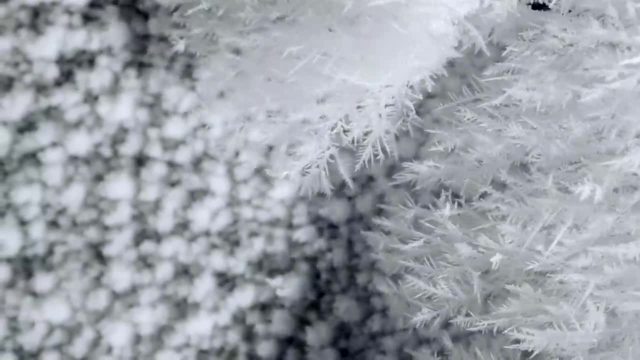 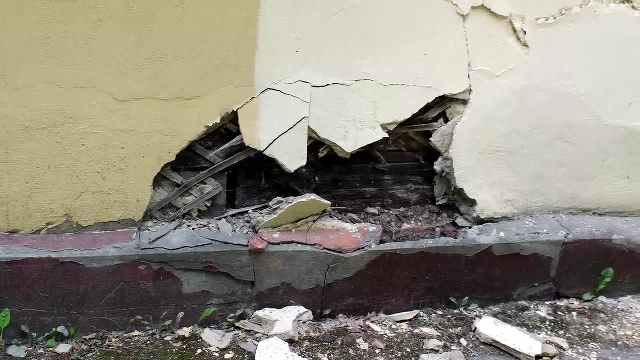 hundreds of times per year. We all know water expands when it freezes and it can do so with prodigious force. When that happens to subsurface water below a structure, it can behave like a jack to lift it up. Over time, these cycles of freeze and thaw can slowly 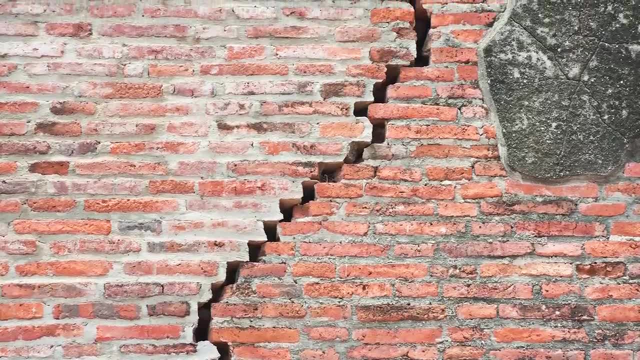 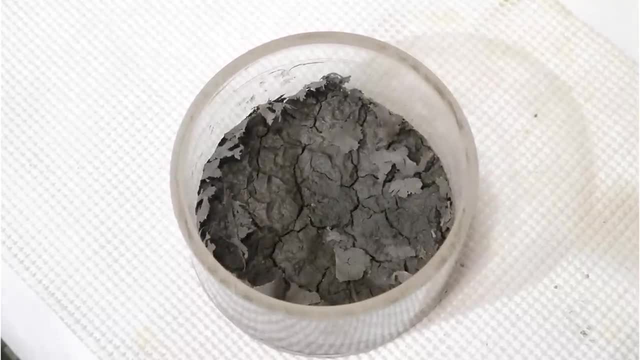 shift or raise parts of a structure more than others, creating issues. Similarly, some kinds of soil expand when exposed to moisture. I also have a video on this phenomenon, so you have two videos to watch after this one. Expansive clay soil can create the same type of damage. 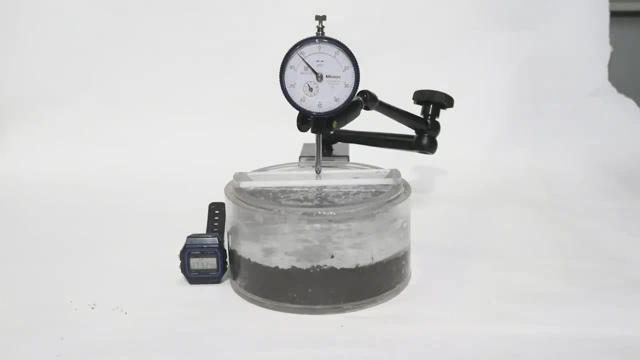 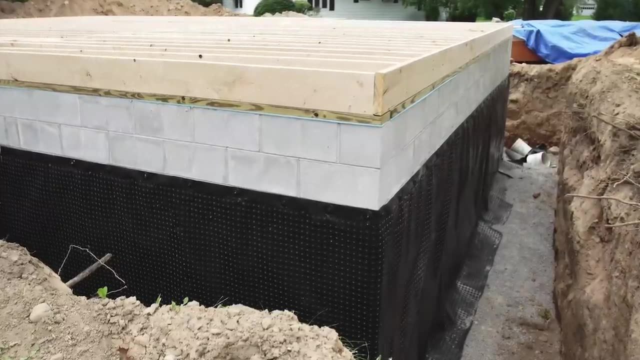 as cycles of freeze and thaw, by subtly moving a structure in small amounts with each cycle of wet and dry. So job number four of a foundation is to reach a deep enough layer that can't freeze or that doesn't experience major fluctuations in moisture content to avoid 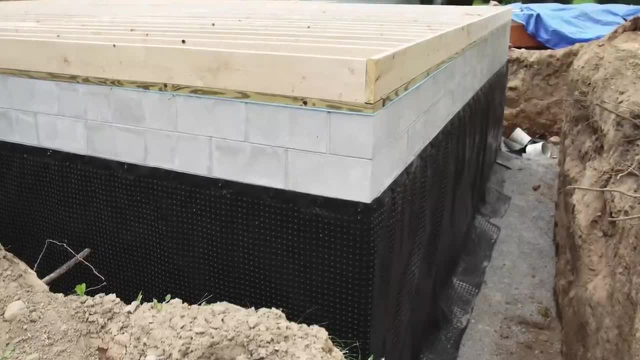 these problems that come with water in the subgrade below a structure. Job number five isn't necessarily applicable to most buildings, but there are many types of structures, like bridges and ponds, that can cause a lot of damage to the structure. So if you have a 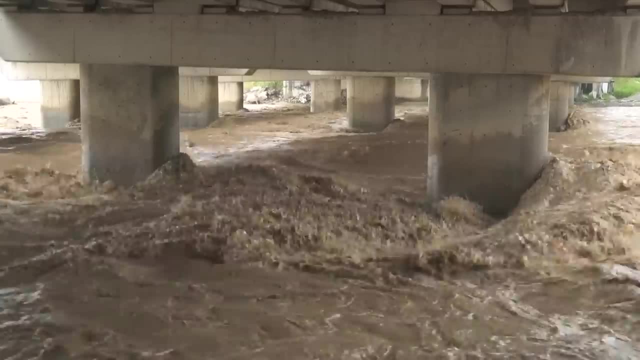 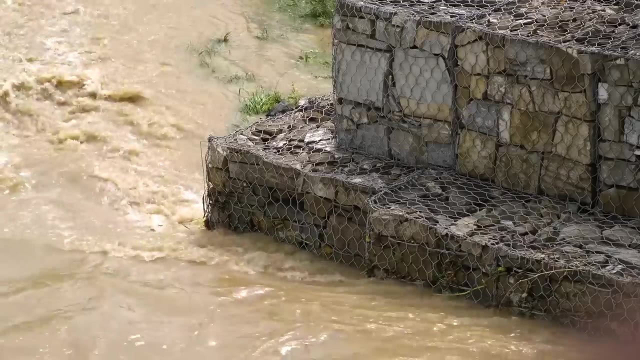 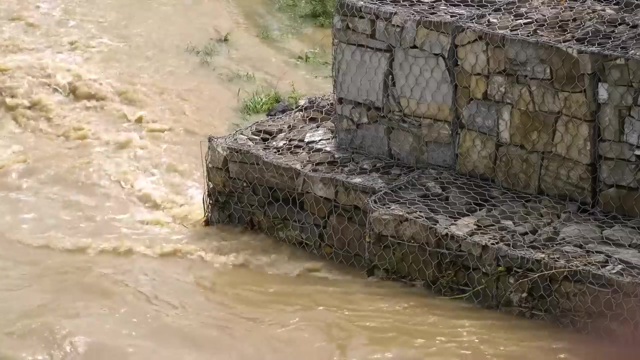 building that doesn't have walls and retaining walls that are regularly subject to flowing water. over time, or sometimes over the course of a single flood, the water can create erosion undermining the structure. Many foundations are specifically designed to combat erosion, either with hard armoring or by simply being installed so deep into the earth that they 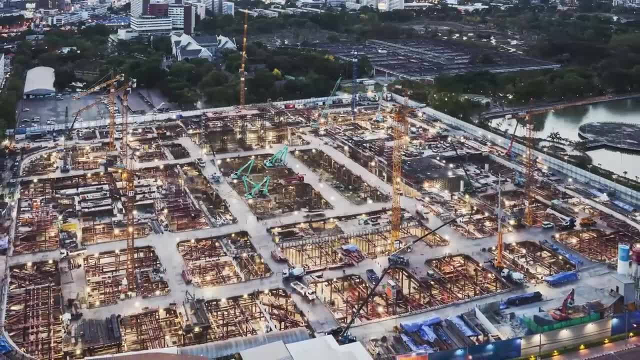 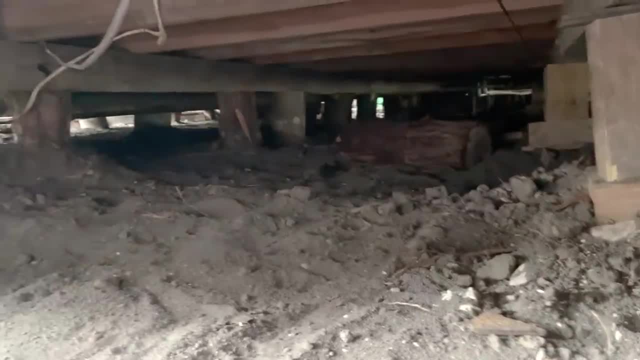 can't be undermined by quickly flowing water. Job number six really applies to all of engineering. Foundations have to be cost-effective. Could the contractor who built my house in the 1940s pay twice as many piers, each one to three times the depth? Of course it can be done. 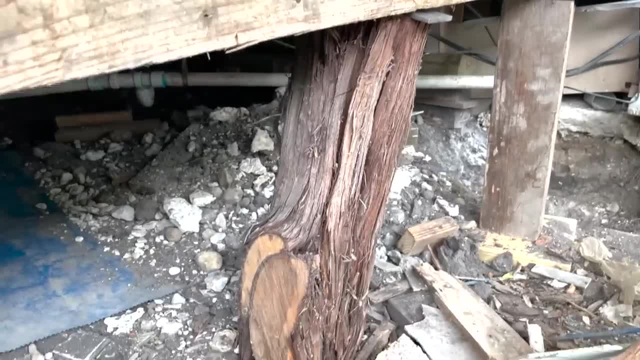 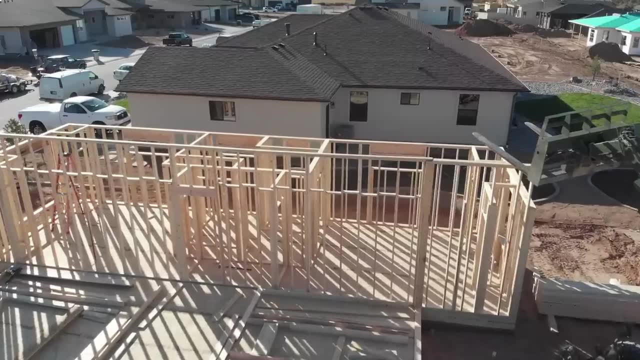 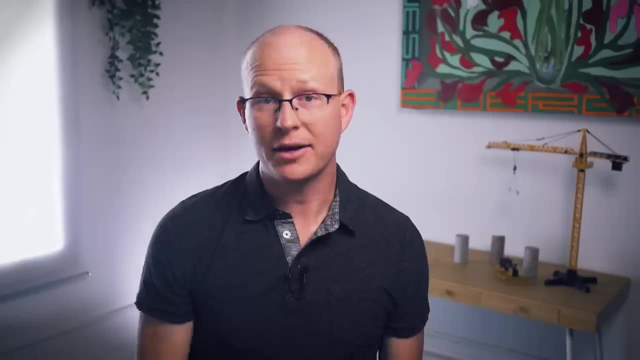 but with some minor maintenance and repairs. this one lasted seventy-five years before needing to be replaced With the median length of home ownership somewhere between five and fifteen years. few people would be willing to pay more for a house with five hundred years of remaining life in the foundation than they would for one with thirty. I could. 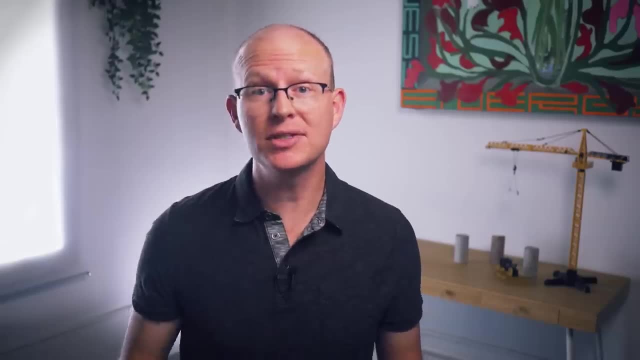 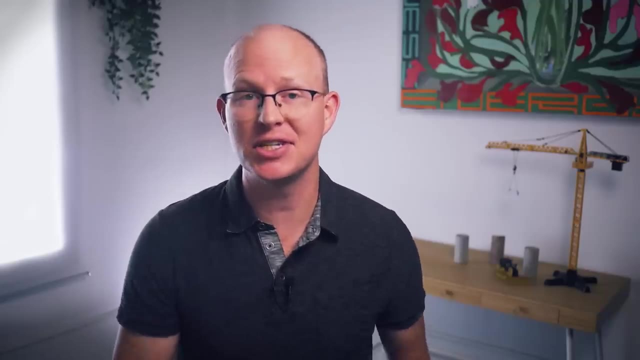 have paid this contractor to build me a foundation that will last hundreds of years, but I didn't. Engineering is a job of balancing control. I don't know if you've ever heard of a job of balancing constraints, and many of the decisions in foundation engineering come. 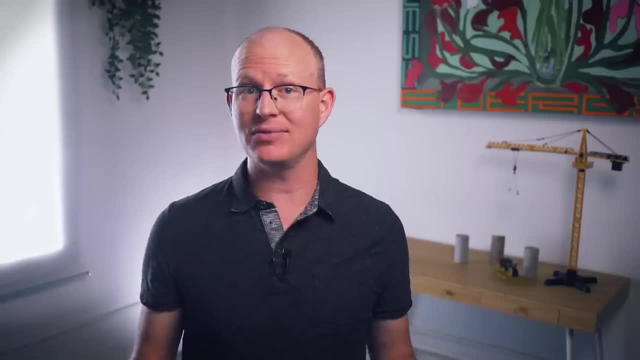 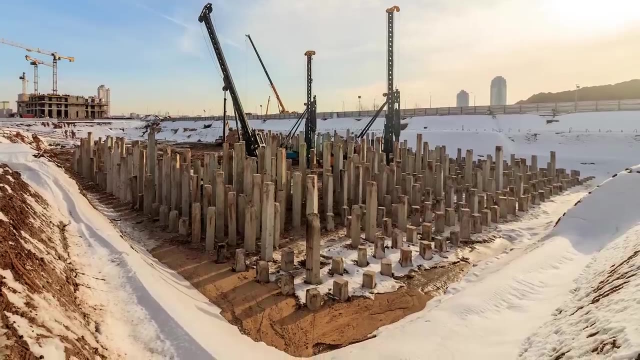 down to the question of how can we achieve all the first five jobs I mentioned without overdoing it and wasting a bunch of money in the process. Let's look at a few ways. Foundations are generally divided into two classes: deep and shallow- Most buildings. 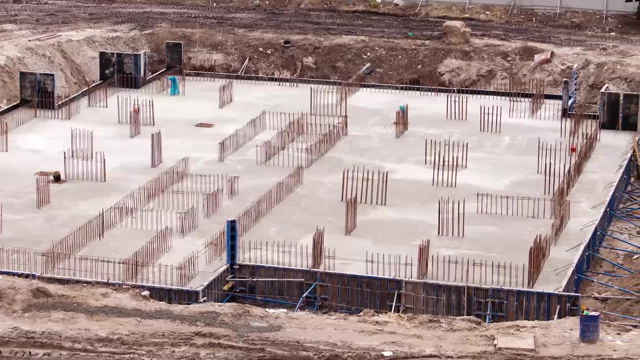 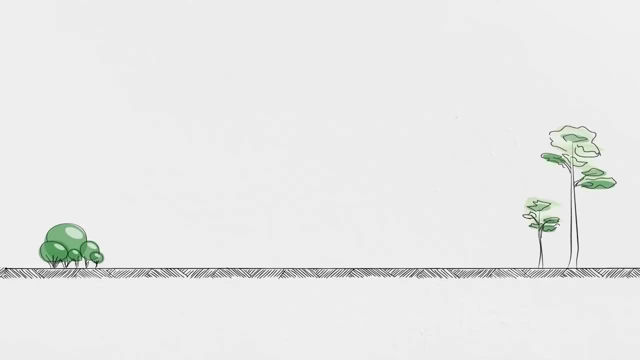 with only a few stories, including nearly all homes are built on shallow foundations. That means they transfer the structure's weight to the surface of the earth or just below it. One of the most basic of these is how my house was originally built. They cut down cedar. 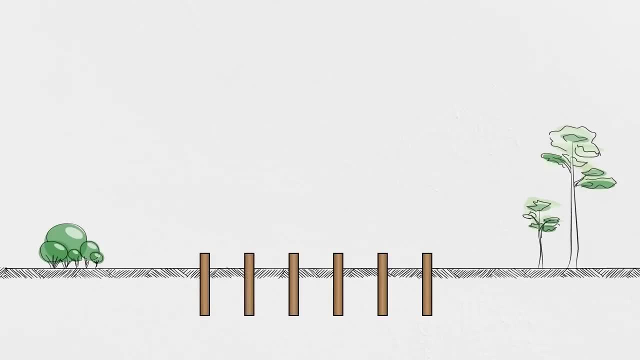 trees, hammered those logs into the ground as piles, laid wooden beams across the top of those piers and then built the rest of the house atop the beams Pier, and beam foundations are pretty common, at least in my neck of the woods, and they have an added benefit. 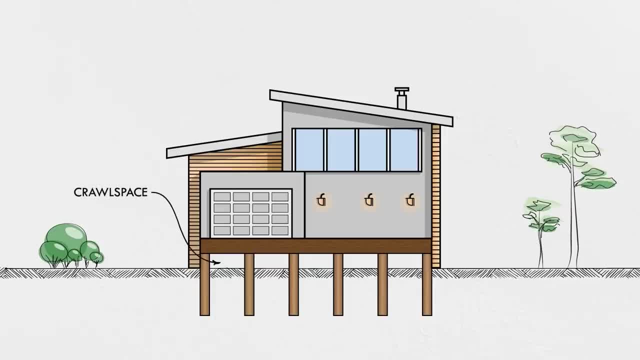 of creating a crawl space below the structure in which utilities like plumbing drains and electric lines can be installed and maintained. However, all these individual, unconnected points of contact with the earth leave quite a bit of space for the structure to be built. 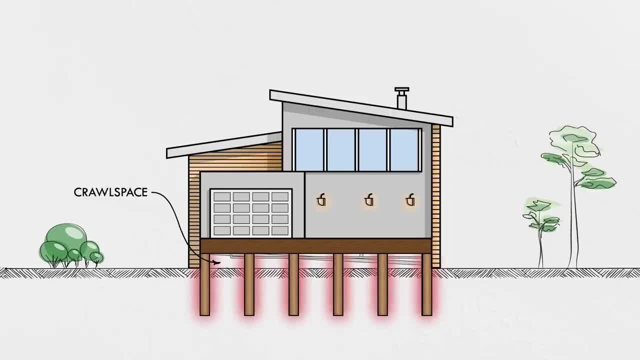 The structure is built on the ground and the walls are built on the ground. The structure is built on the ground and the walls are built on the ground. and the walls are built on the ground. They provide a bit of room for differential movement. 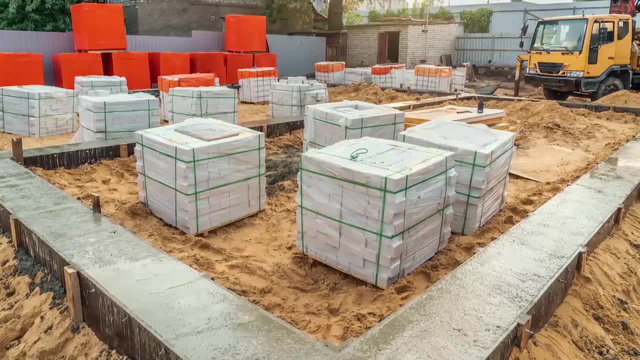 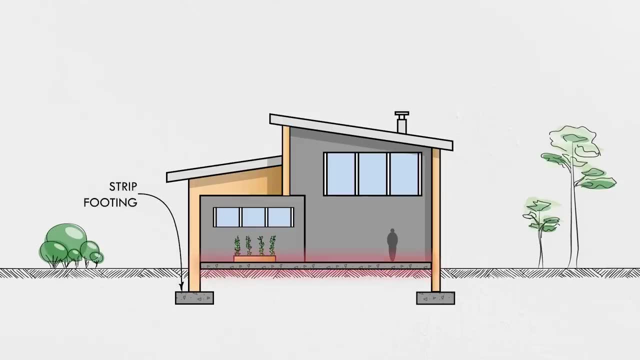 Another basic type of shallow foundation is the strip footing, which generally consists of a ribbon or strip of concrete upon which walls can sit. In some cases the floor is isolated from the walls and it sits directly on a concrete slab atop the subgrade, But strip footings can also support floor joists making room. 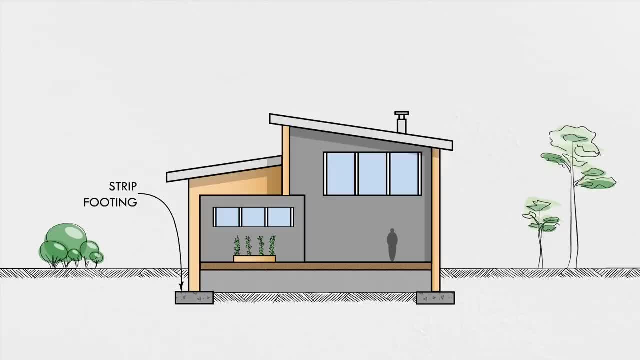 for a crawl space below. For sites with strong soils, this is a great option because it's simple and cheap. But if the subgrade soils are poor, strip footings can still allow differential movement. walls aren't rigidly connected together. In that case, it makes sense to use a raft foundation. 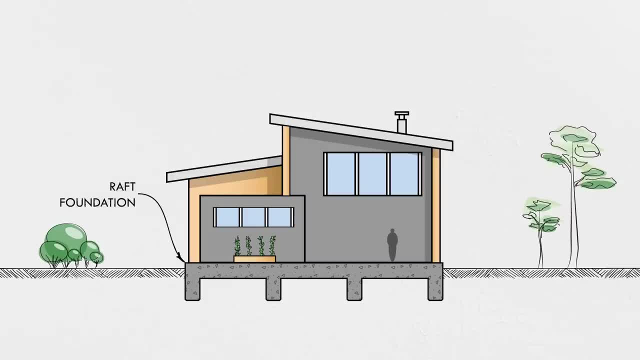 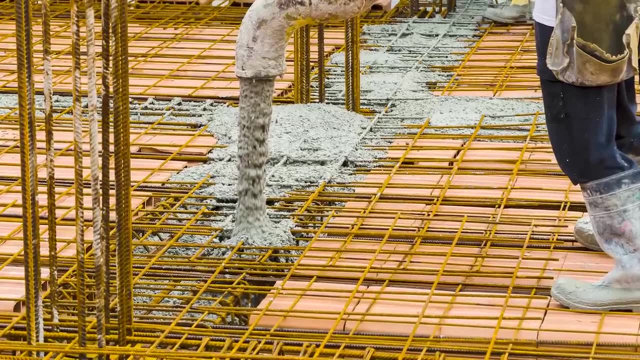 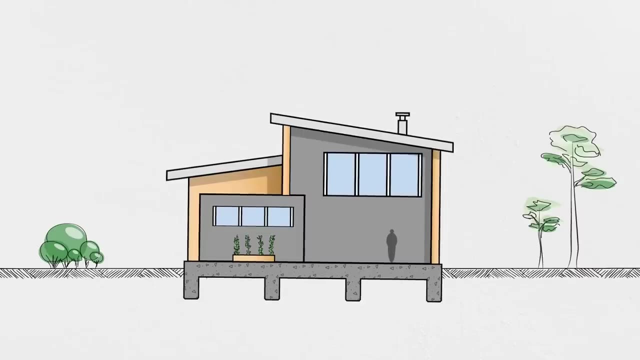 a completely solid concrete slab that extends across the entire structure. Raft foundations are typically concrete slabs placed directly on the ground, usually with some thickened areas to provide extra rigidity. They distribute the loads across a larger area, reducing the pressure on the subgrade, and they can accommodate some movement. 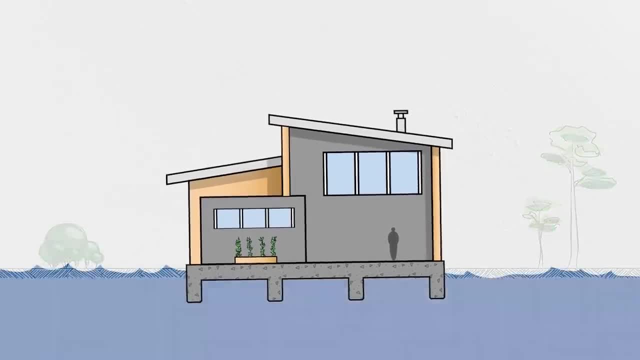 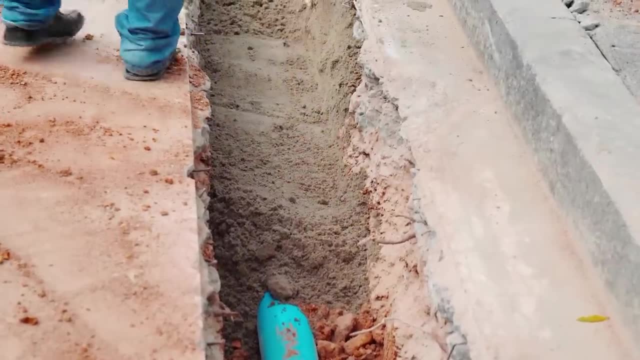 of the ground without transferring the movement into a structure, essentially riding the waves of the earth like a raft on the ocean. hence the name. However, they don't have a crawl space, which makes plumbing repairs much more challenging. One issue with all shallow: 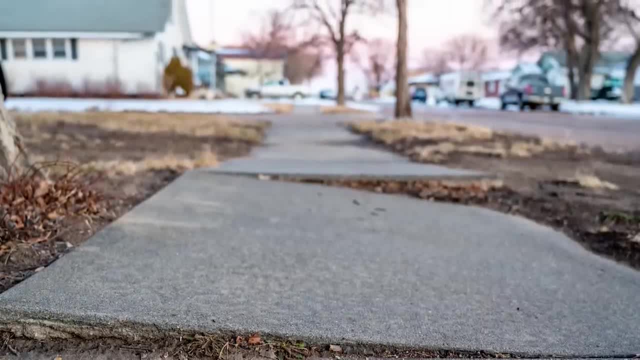 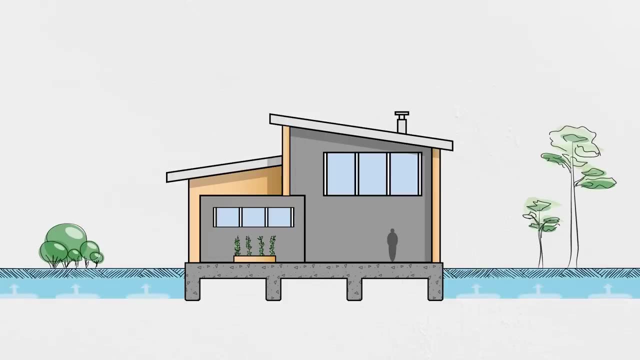 foundations is that you still need to install them below the frost line. that is the maximum depth to which water in the soil might freeze during the harshest part of the winter, in order to avoid frost heaving. In some parts of the contiguous United States, the frost line can be upwards of. 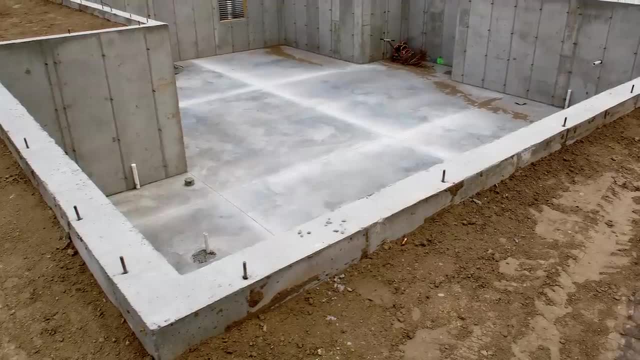 eight feet or nearly two and a half meters. If you're going to dig that deep to install a foundation anyway, you're going to need a lot of work to do that. If you're going to dig that deep to install a foundation anyway, you're going to need a lot of work to do that. If you're going to dig that deep to install a foundation anyway- you're going to need a lot of work to do that- You might as well just add an extra floor to your structure below the ground. That's usually called a basement and it can be considered a building's foundation. 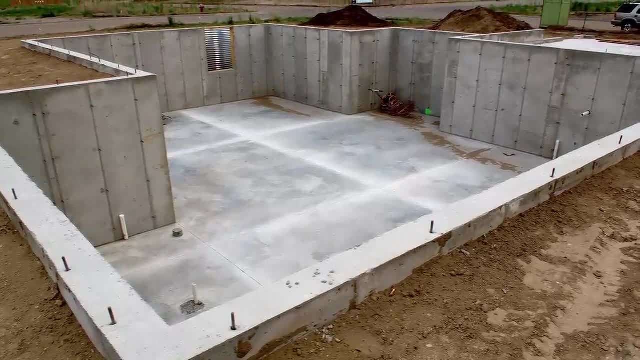 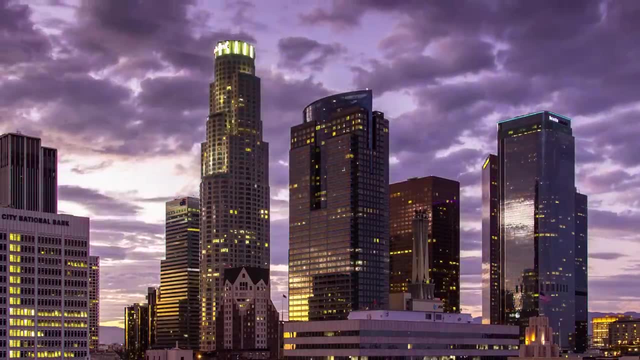 although the walls are usually constructed on a raft or strip footings as described above. As a structure's size increases, so do the loads it imposes on the ground, and eventually it becomes infeasible to rely only on soils near the surface of the earth. 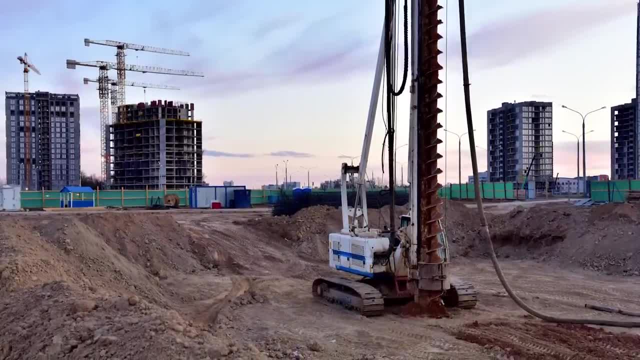 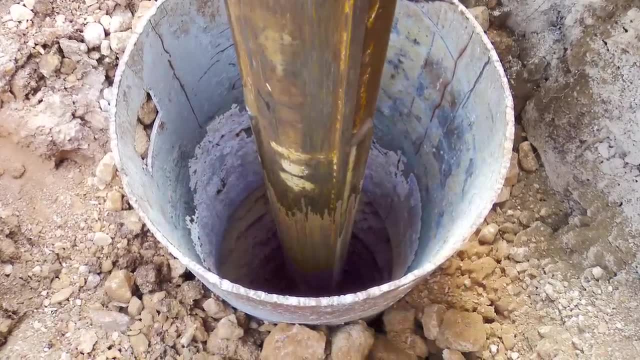 Tall buildings, elevated roadways, bridges and coastal structures often rely on deep foundations for support. This is especially true when the soils at the surface are not as firm as the layers farther below the ground. Deep foundations almost always rely on piles, which are vertical structural elements that 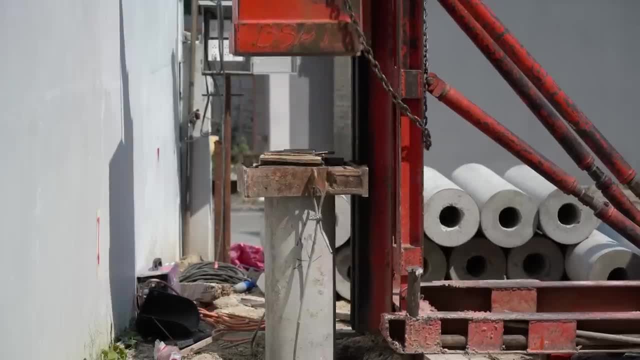 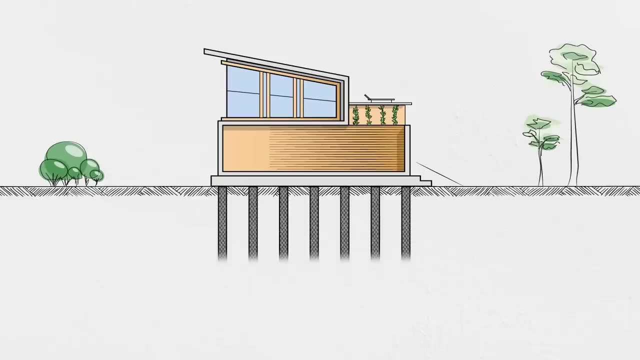 are driven or drilled into the earth, often down to a stronger layer of soil or bedrock, And there are way more types than I could ever cover in a single video. Piles not only transfer loads at the bottom, called inbaring. 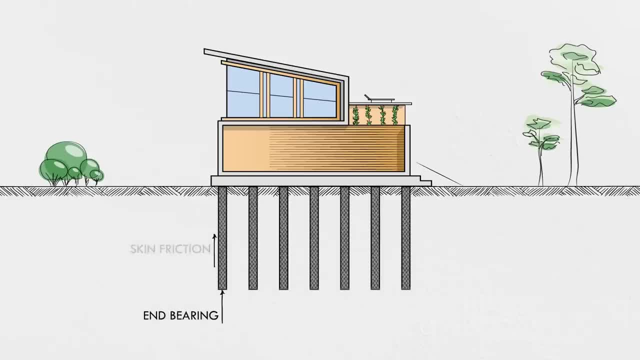 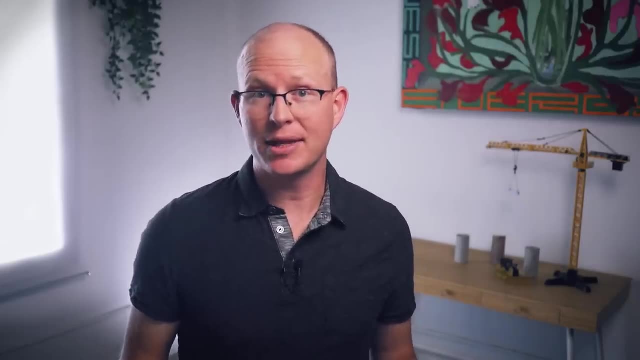 but they can also be supported along their length through a phenomenon called skin friction. This makes it possible for a foundation to resist much more significant loads, whether downward, upward or horizontal, within a given footprint of a structure. One of the benefits of driven piles is that you install them in somewhat the same way they'll be loaded in their final configuration. 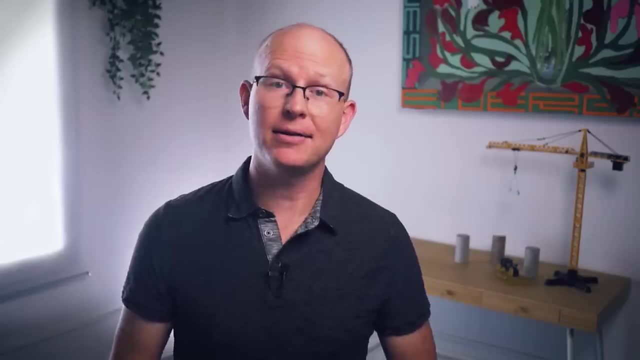 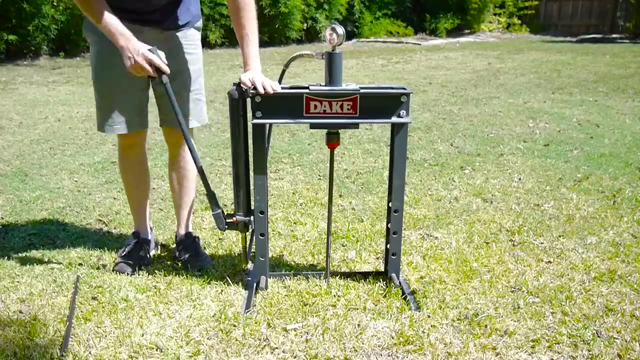 There's some efficiency there, because you can just stop pushing the pile into the ground once it's able to resist the design loads. There is a problem with this, though. Let me show you what I mean. This hydraulic press has more than enough power to push the steel rod into the ground. 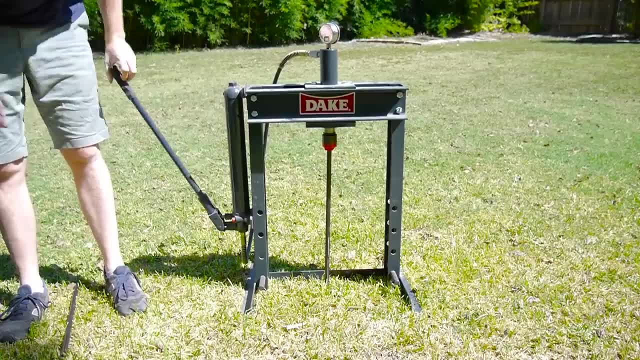 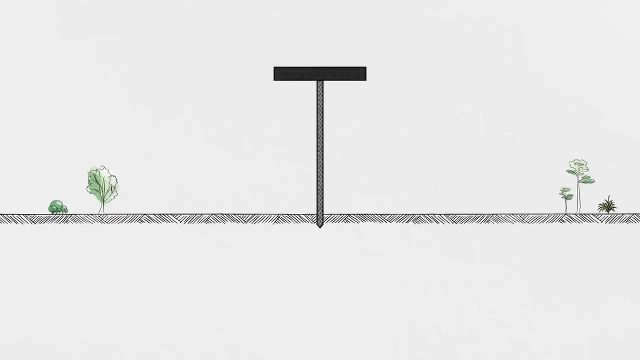 and at first it does just that. but eventually it reaches a point where the weight of the press is less than the bearing capacity of the pile and it just lifts itself up Easy, you might think, Just add more weight. But consider that these piles might be designed to support the weight of an entire structure. 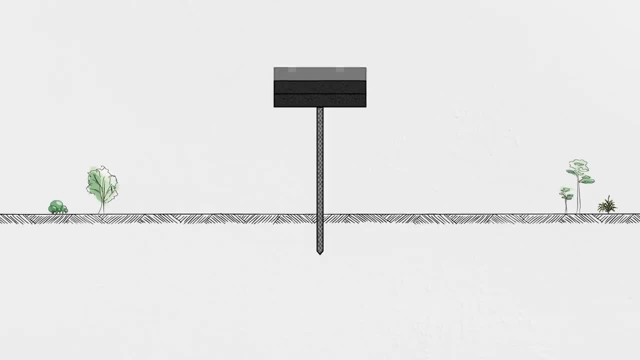 It's not feasible to bring in or build some massive weight just to react against to drive a pile into the ground. Instead, we usually use hammers, which can deliver significantly more force to drive a pile with only a relatively small weight. The problem with hammered piles is that the dynamic loading they 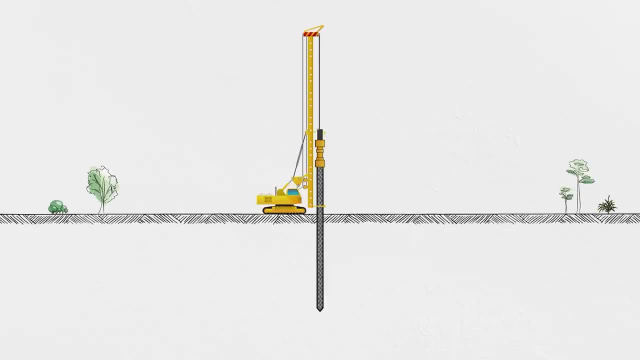 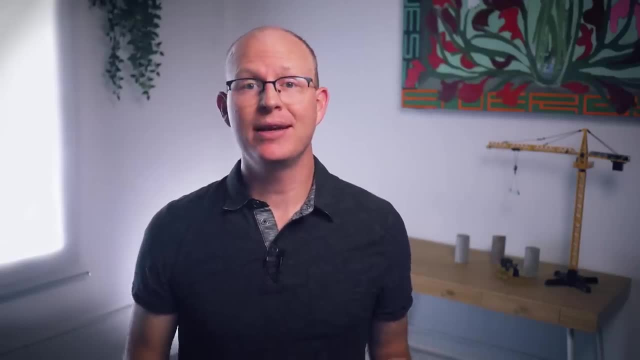 undergo during installation is different from the static loading they see once in service. In other words, buildings don't usually hammer on their foundations. For example, if a pile can withstand the force of a 5-ton weight dropped from 16 feet or 5 meters without moving, what's the equivalent static load it can withstand? 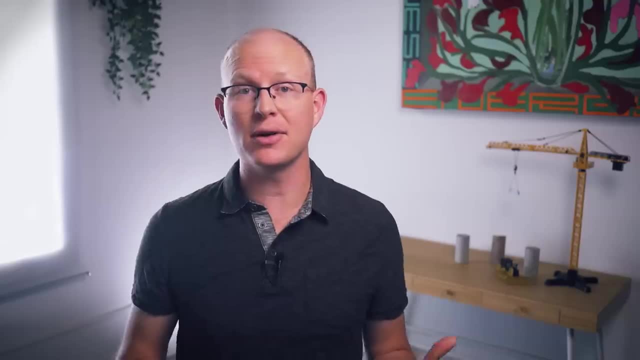 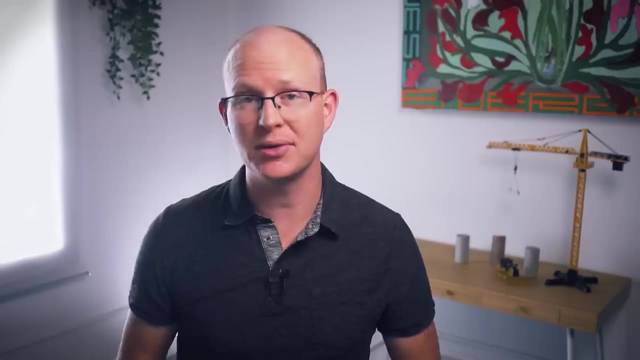 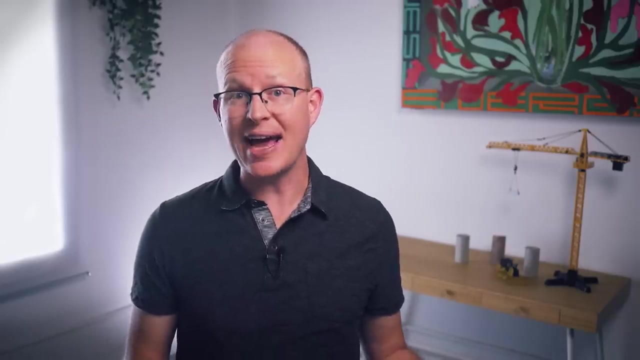 That turns out to be a pretty complicated question, And even though there are published equivalencies between static and dynamic loads, their accuracy can vary widely depending on soil conditions. That's especially true for long piles, where the pressure wave generated by a hammer might not even travel fast enough to load the entire member at the same moment in time. Static tests are more reliable but also more expensive, because you either have to bring in a ton or thousands of tons of weight to put on top, or you have to build additional piles with a beam across them to give the test rig. 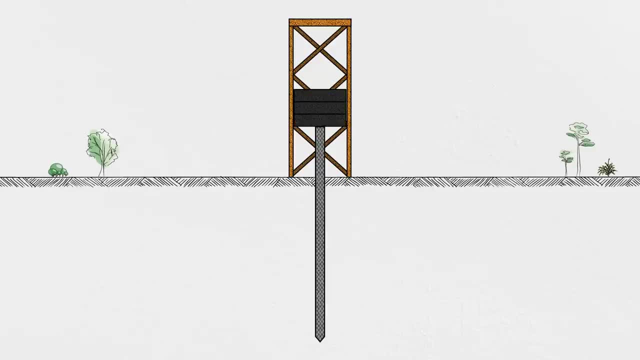 something to react against. One interesting solution to this problem is called statnamic testing of piles. In this method, a mass is accelerated upward using explosives, creating an equal and opposite force on the pile to be tested. It's kind of like a reverse hammer. 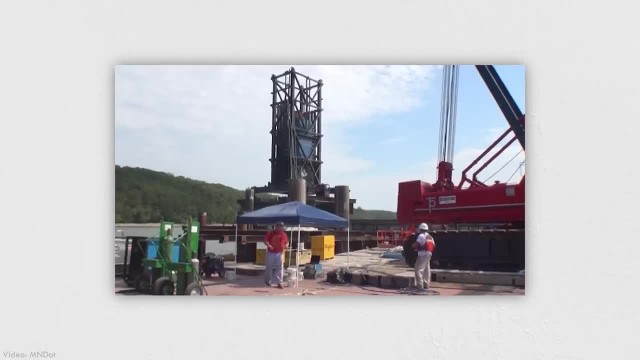 except, unlike a hammer, where the force on the pile lasts only for a few milliseconds. the duration of loading in a statnamic test is often upwards of 100 or 200 milliseconds. That makes it much more similar to a static force on the pile, without having to bring 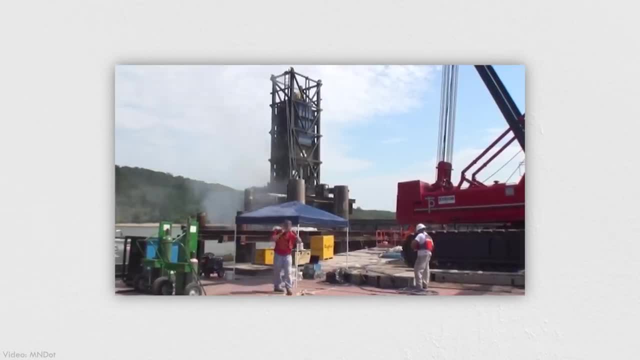 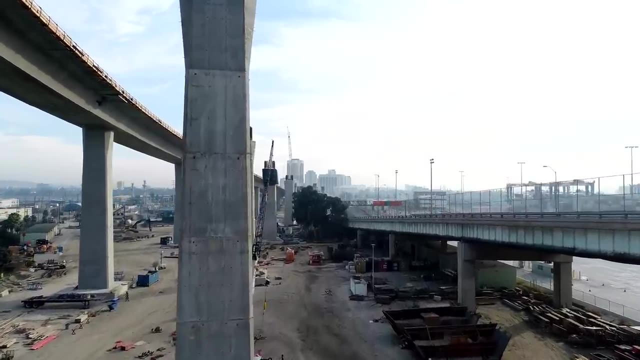 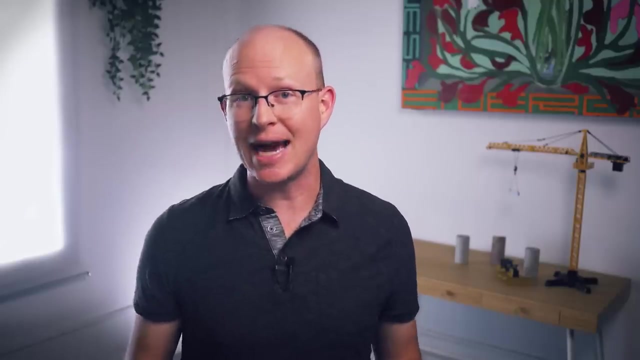 in tons and tons of weight or build expensive reaction piers just to conduct a test. I'm only scratching the surface or subsurface of a topic that fills hundreds of engineering textbooks and the careers of thousands of contractors and engineers, If all the earth. 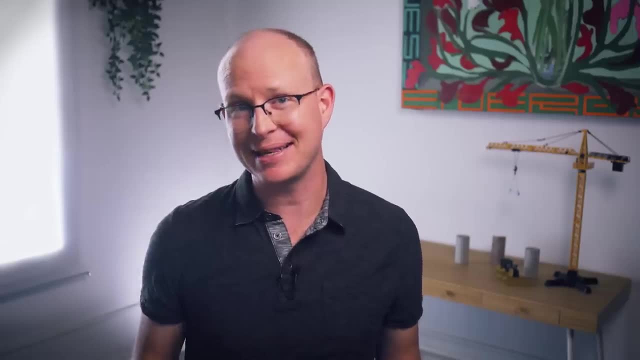 was solid rock, life would be a lot simpler, but maybe a lot less interesting too. If there are topics and foundations you'd like to learn more about, add a comment or send me an email and I'll try to address it in a future video, but I hope this one gives you some appreciation of 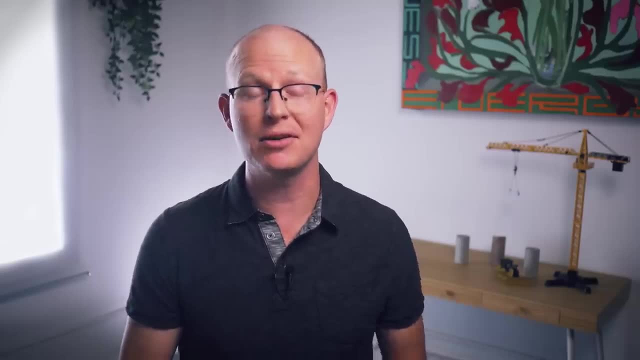 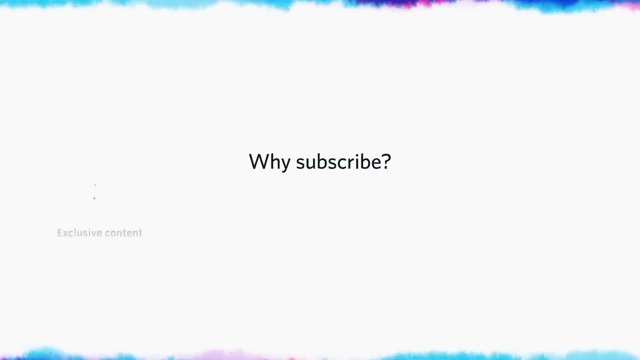 those interesting topics. Thanks for watching and I'll see you next time. Hey, thanks for sticking around to the end of this video. You know how this works because you probably watch a lot of videos about science and engineering to the end, just like I do. 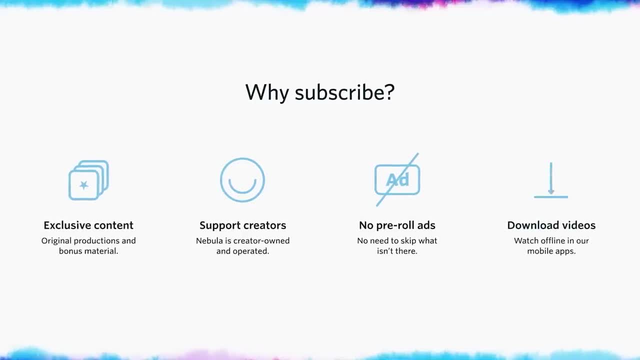 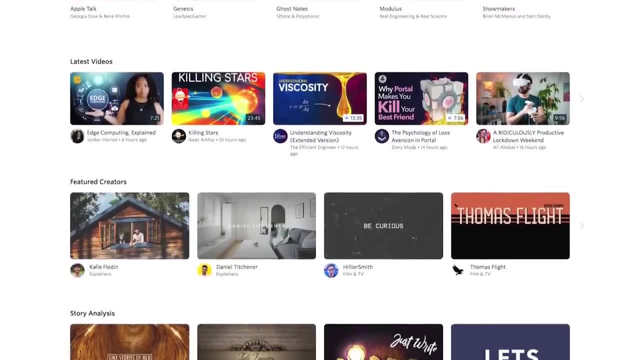 You probably also don't enjoy watching ads like this one, which is great, because Nebula doesn't have any. Nebula is a streaming service built by and for independent creators like MinutePhysics, Real Engineering, Wendover Productions and a bunch of others, including me. It's a way for us. 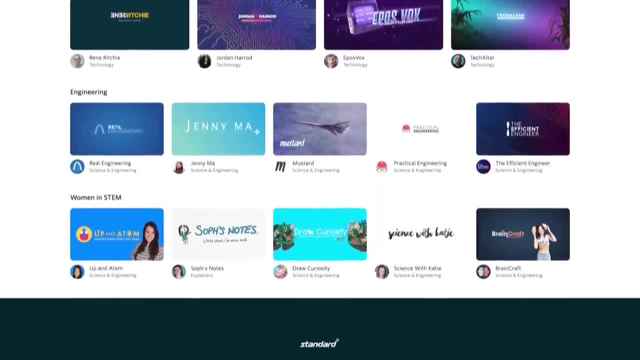 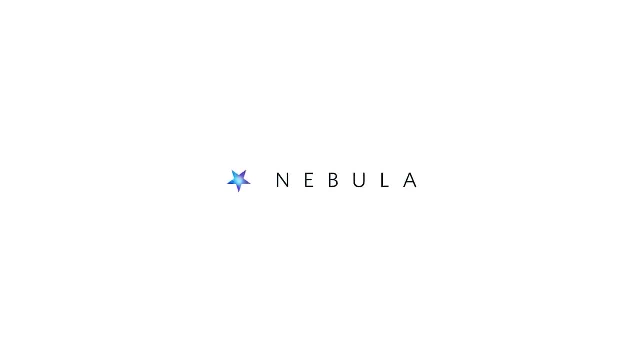 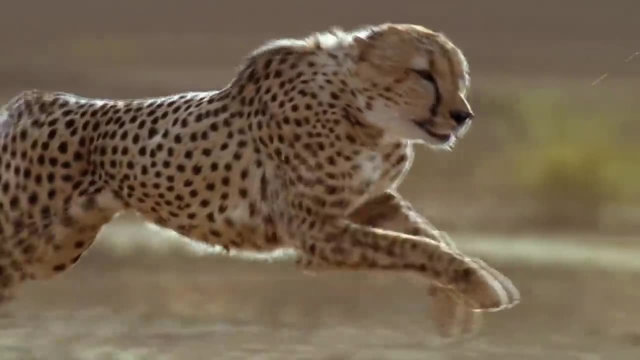 to share ideas that might not work on advertiser-supported platforms like YouTube. My videos go live there the day before they publish here with no ads or sponsorships, And we're super excited to continue our partnership with CuriosityStream, a service with thousands of documentaries and non-fiction titles on pretty much every subject you can imagine. 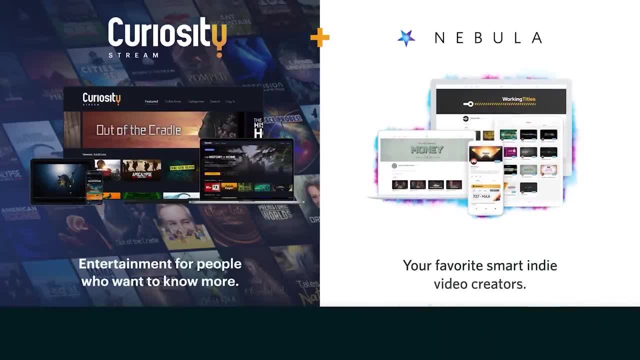 CuriosityStream loves independent creators and wants to help us grow our platform, so they're offering free access to Nebula when you sign up at curiositystreamcom. slash practicalengineeringcom- I know there are a lot of streaming services right now- and all those monthly subscriptions. 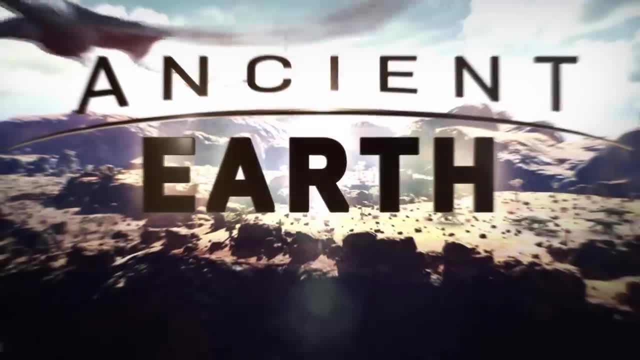 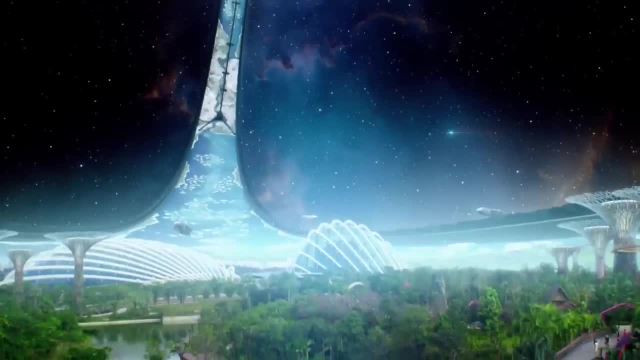 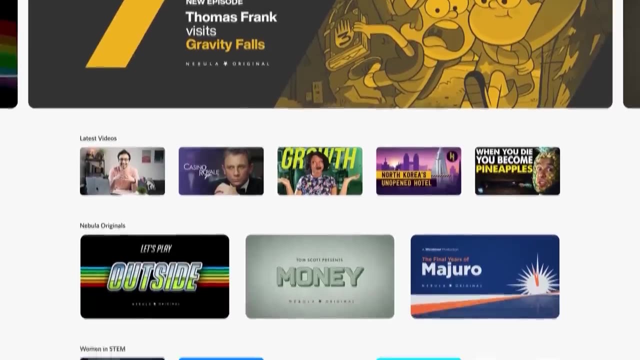 can be tough to keep track of. That's why this bundle is such an awesome deal. CuriosityStream's taking 26% off an annual plan That makes it only $15 for an entire year of access to thousands of thought-provoking documentaries on CuriosityStream and everything on Nebula as well. I love watching. 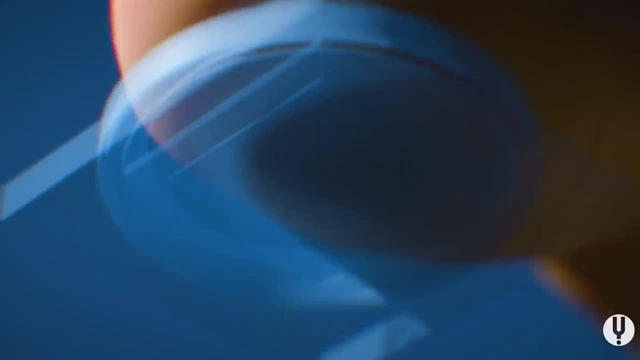 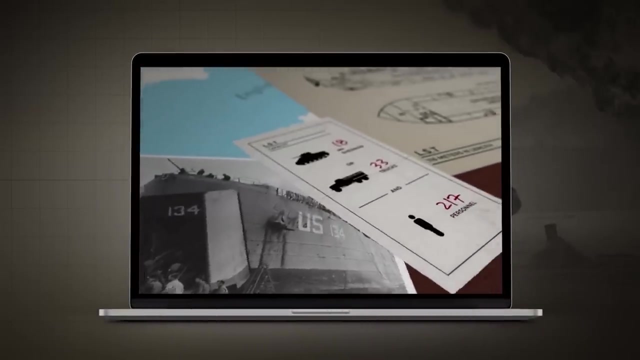 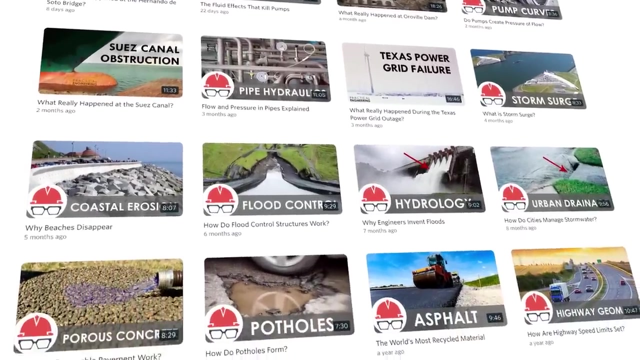 the European Inventor Awards that showcase the coolest new inventions each year on CuriosityStream. or watch the Nebula-exclusive series Logistics of D-Day by my friend Brian at Real Engineering. It's a great way to support my channel and a whole host of your other favorite educational creators. Plus, it's just a great deal. 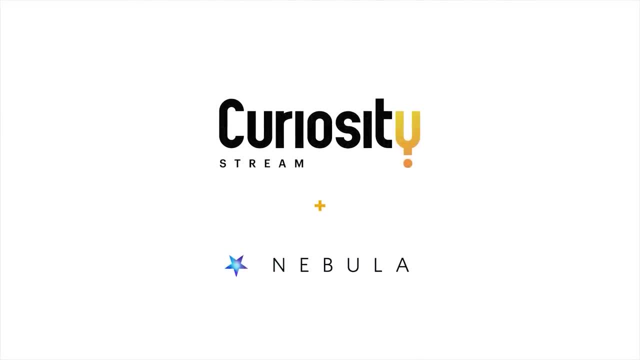 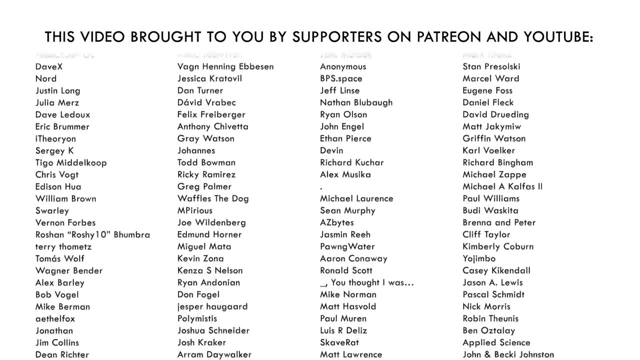 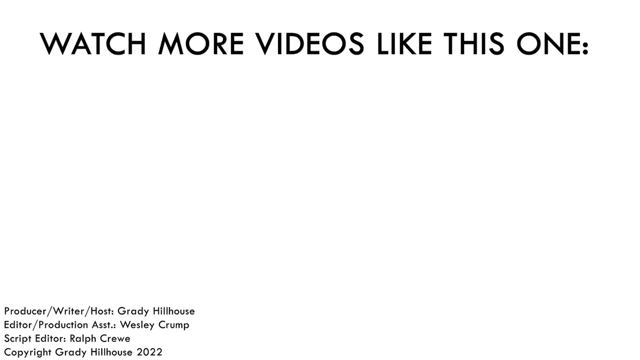 Do us both a favor and click that link in the description. Thank you for watching and let me know what you think. I'll see you next time.